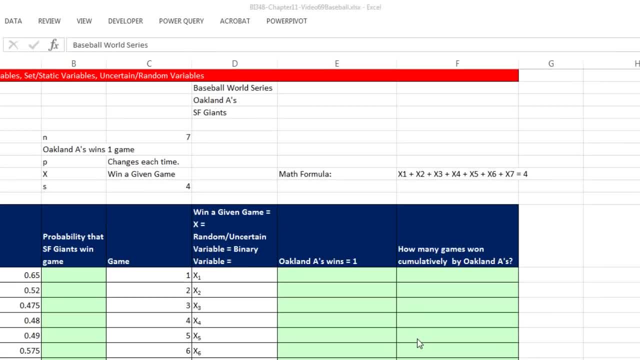 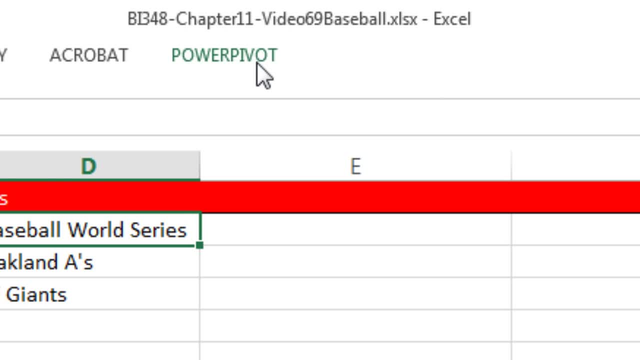 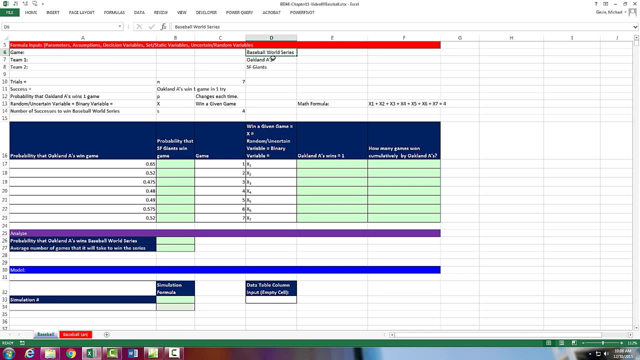 Welcome to Highline BI348 class, video number 69.. Hey, if you want to download this workbook BI348, chapter 11,, video 69, and follow along, click on the link below the video. Hey, this is our last video in our simulation chapter, chapter 11, and it's our last video for this BI348 class, and we have a great example. 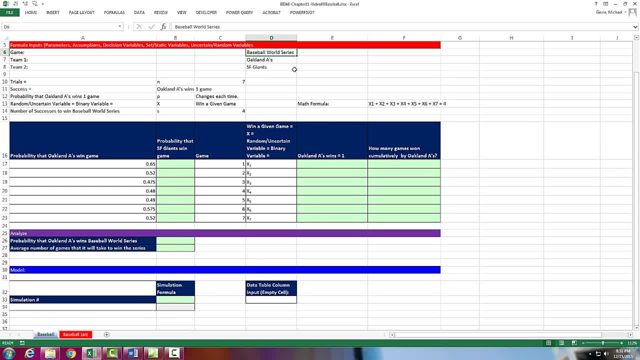 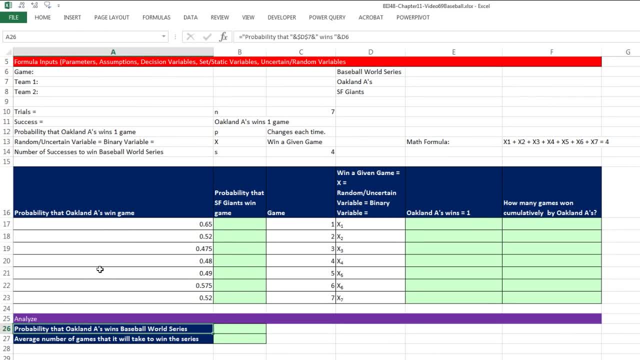 We have a baseball World Series example for how to use simulation. Now the A's and the San Francisco Giants are going to be playing and our goal is to calculate the probability that the Oakland A's will win the baseball World Series and calculate the average number of games that it will take to win the series. 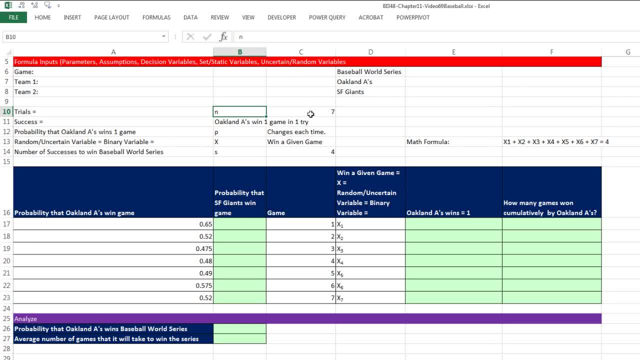 Now here's some of our variables up here: Trials, and that's seven World Series games. We'll define a success as Oakland A's win one game in one try. Probability that A's win one game. well, it changes each time. Look at this: .65, .52, .475, .48, so we can't use a binomial experiment. 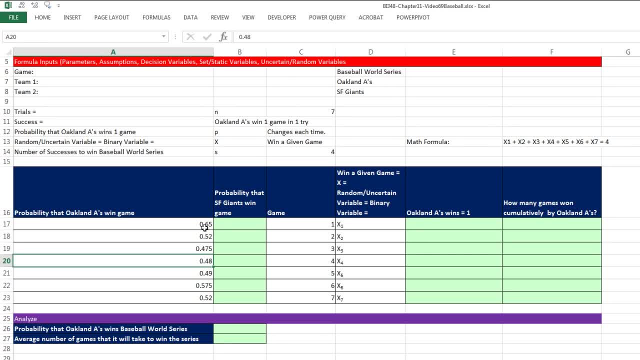 Now these probabilities, where do they come from? Well, if it's the Oakland A's, you know, Billy Bean and his statistics pals put a lot of time and effort into calculating each one of these Things like starting pitchers, math Matchups, heating, on-base percentage, home field advantage and many other variables. 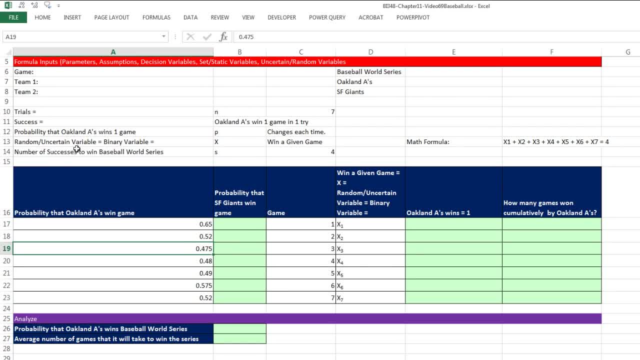 But each one is different. Our random, uncertain variable will be a binary variable, X. it'll be just that the A's win a given game. Number of successes to win the baseball World Series. well, you need a total of four. Alright, I'm going to calculate the complement here, even though we really don't need it. 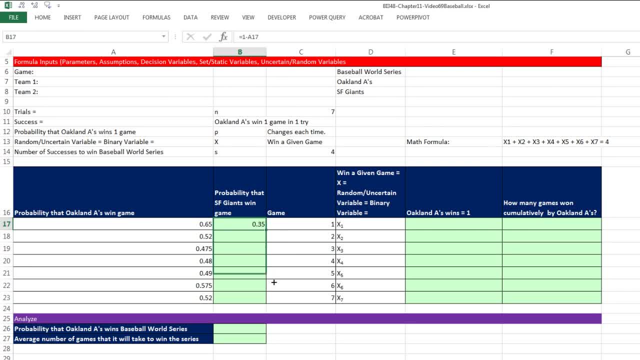 That's the probability that the Giants win. The Giants will win any one of these particular games. And now here's X1 to X7, so we're going to have seven different variables in a random Zero, or one for each one of these games. 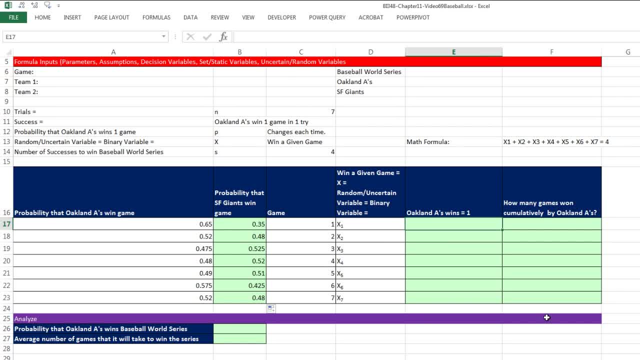 Zero means they didn't, the A's didn't win, One means they win. So we're going to use equals, the IF function, and we've used the RAND function many times in Chapter 11 here for simulation. The RAND is an argument-less function that will calculate a number between: 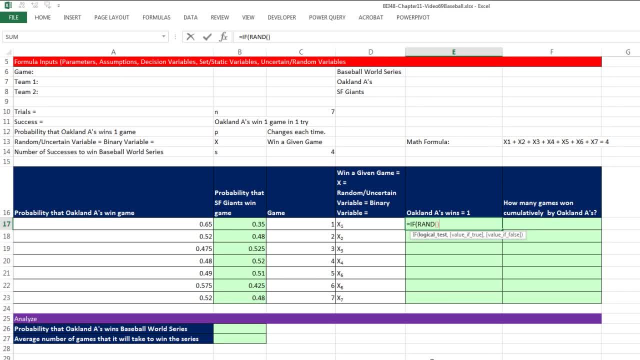 zero and one. And I'm going to ask the question: hey, random probability of winning, are you greater than the probability that we think the A's will win? If it's greater than that, then we'll say comma for value of true zero. 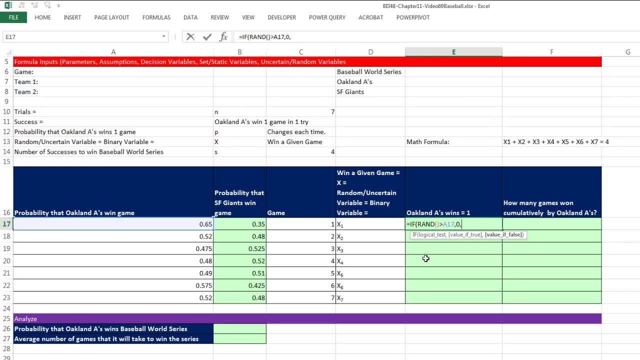 That means the A's did not win, Otherwise one. they won. Close parentheses control, enter, Double click and send that down. Now if I hit the F nine key to randomize, you can see we get a different set of zeros and ones. 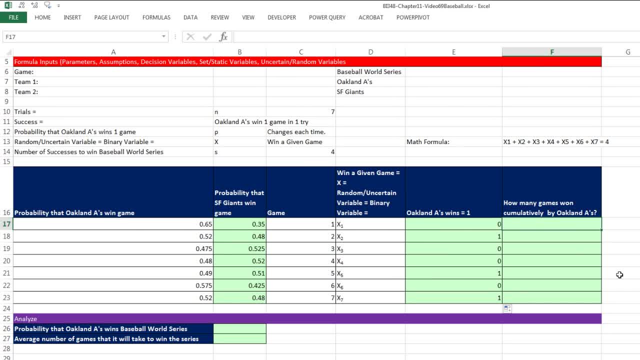 A's lose or A's win. Now I need to calculate the cumulative total. So down here it should be one, when we get down here it should be two, and finally it should be three. So I use equals, the SUM function, And I need to say E17, colon, close parentheses. 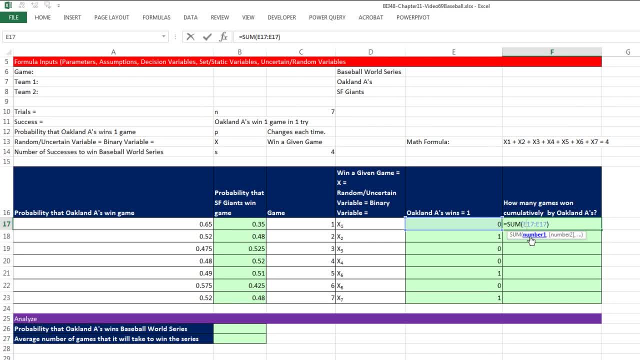 We need an expandable range here. so I'm going to put my cursor and touch the first E17. F4 to lock it. That expandable range control. enter and copy it down. Any particular cell you can see, sure enough. 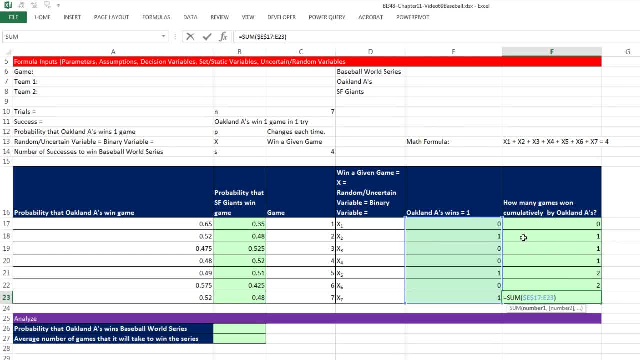 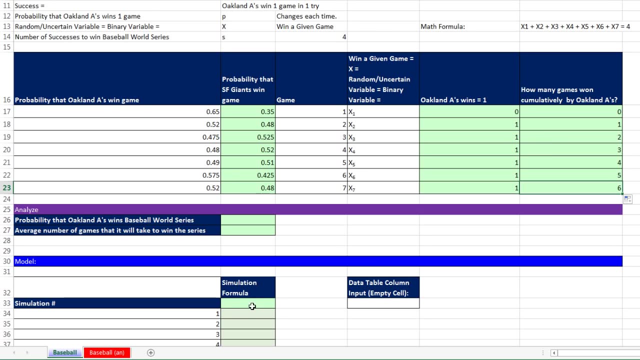 the SUM function is expanding and adding the total games that the A's have won cumulatively. Now, if I hit F9, you can see there it is: Four wins mean they won the World Series in game five. Now we want to come down here and think about a simulation formula. 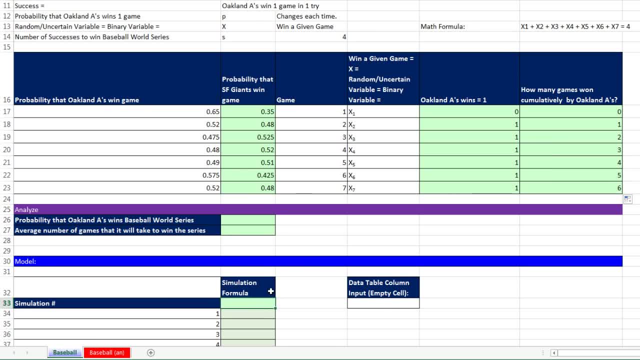 because again we have to answer both of these questions And I'm going to get a little trickier. I'm just going to look up four within this range right here, using the MATCH function, Equals. MATCH is a lookup function. The lookup value will be. I'm looking up four. 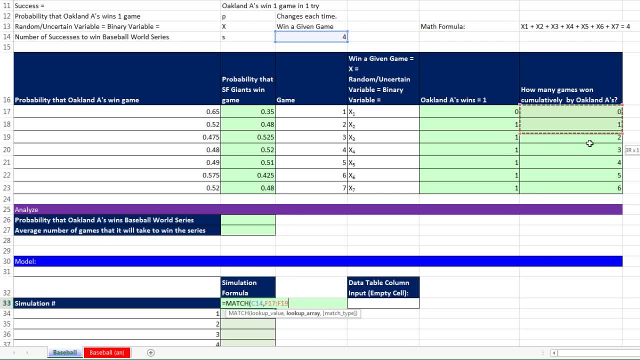 comma within this lookup array. right here, comma And we need to use exact match. Now, the advantage and the beauty of exact match for this example is that if there are duplicates over here, because sometimes our formula will show four, four, four- 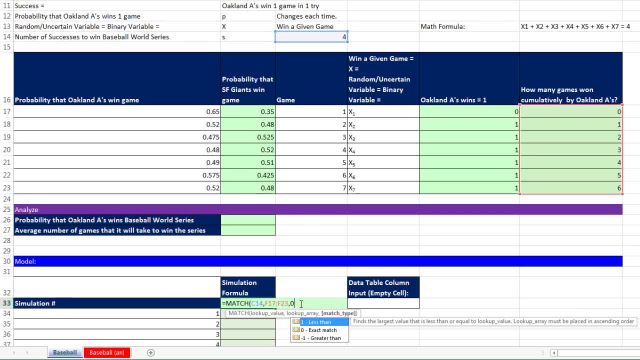 it will only pick up the relative position of the first number four. So again, MATCH will look through a range and tell you the relative position of the item it's looking up. That means the number four. So when I control enter right now. look at that. 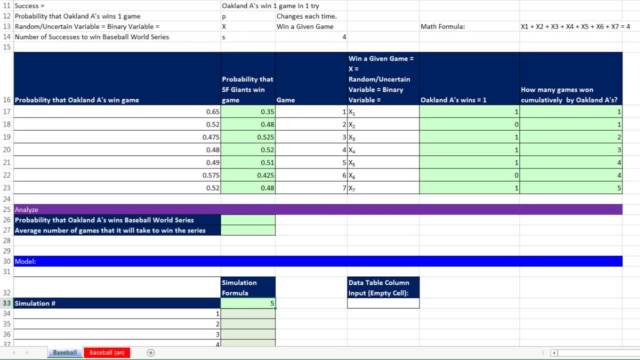 MATCH found one, two, three, four, five. So the A's won in the fifth Game of the World Series And the MATCH function is never going to report the wrong answer because it's only going to find the first number. four, because we have exact match. 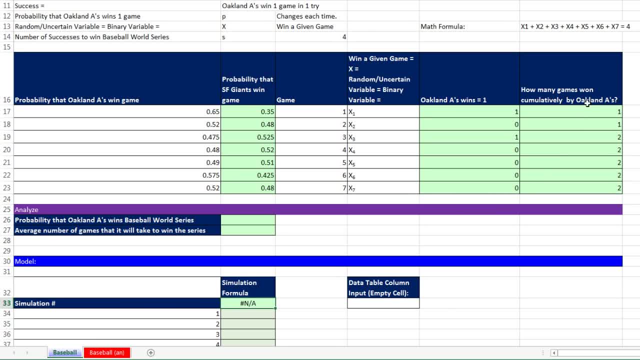 Now, when we hit F9, there will be some cases like this one right here, where MATCH doesn't find a four, That N A is going to mean they didn't win the World Series. Now we want to copy this formula down. We have control down arrow. 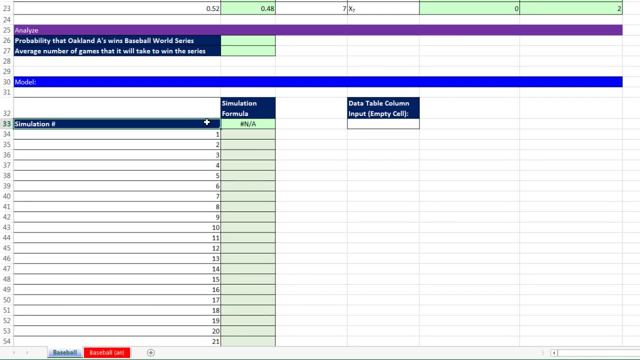 We have our 10,000 simulation numbers There that we're going to need for our formula, or are just sitting there to trick the data table because we're going to copy this formula down? Highlight control. shift down arrow control backspace. 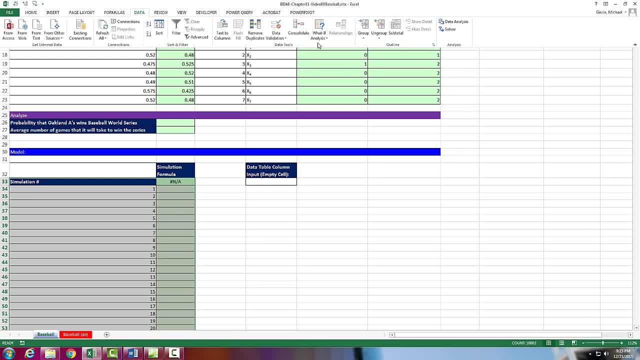 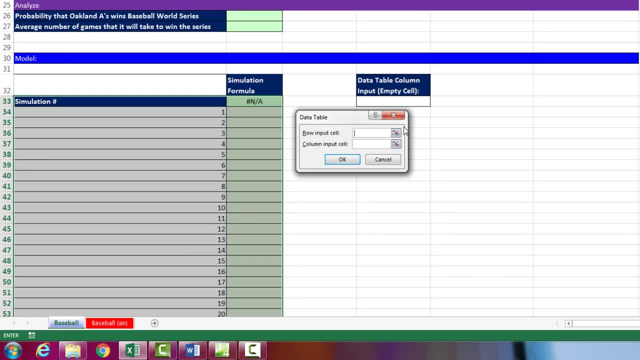 And now, to copy this down, we go to data data tools. what if analysis data table? or we can use the keyboard Alt D, T for data table? We do not have a row input, We have a column input And we're going to trick the data table feature. 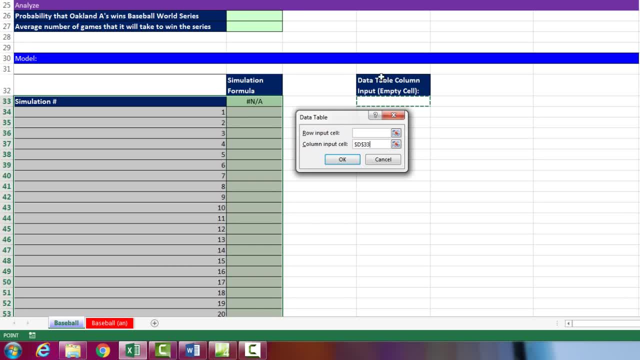 by clicking a number, An empty cell. Now, because this empty cell is not connected to that formula, right there data table will try to substitute each one of these numbers in, But because that formula is not connected, it just won't work. All data table will do. 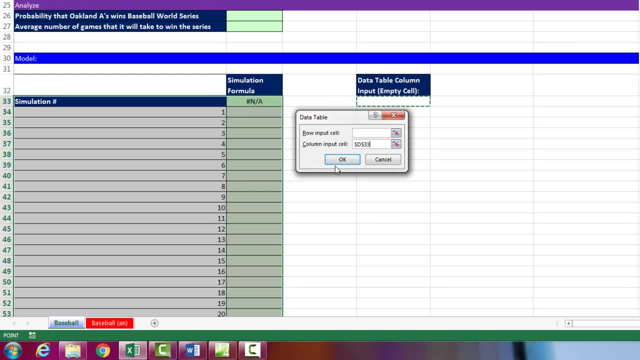 is copy our simulation formula down And when I click OK instantly. Now, as we saw in earlier videos, we use the data table feature because in general it will calculate faster than a formula with lots of randomizing variables in it. Now look at this in our first simulation. 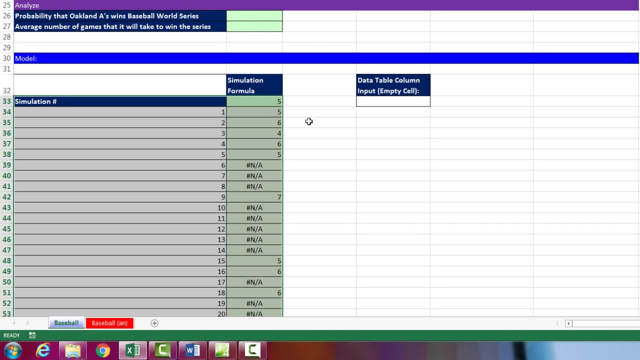 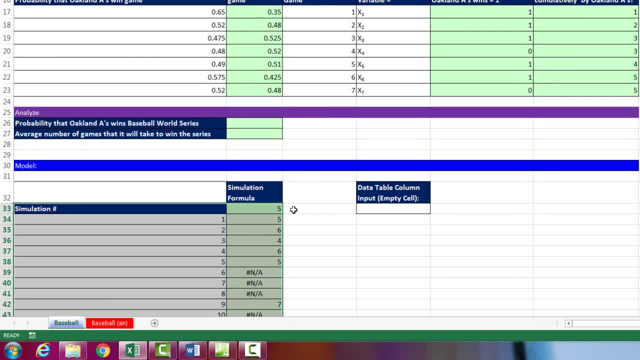 The A's won in five times. Then the second simulation: they won in six times, four times Didn't win, didn't win, didn't win, and so on. Now, how are we going to deal with the N? A's up here? 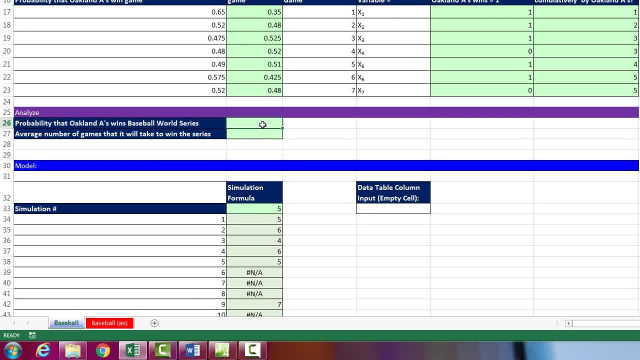 Because we have to calculate probability that the Oakland A's win the World Series And then average number of games it took. Well, let's first do the probability that the Oakland A's win the Baseball World Series. I'm going to actually use the COUNT function. 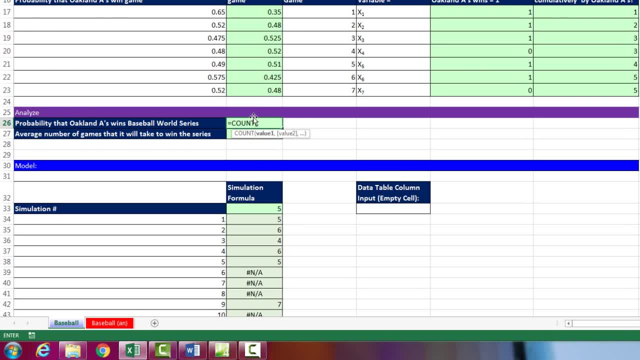 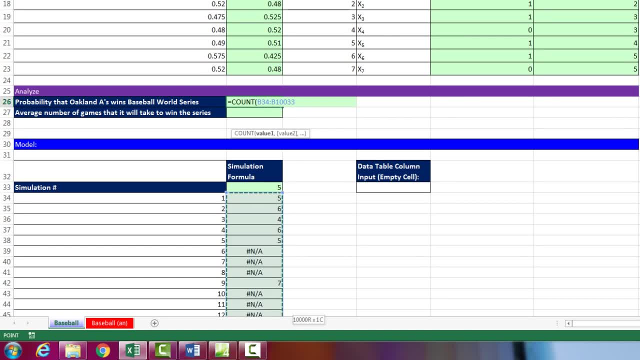 Now the COUNT function is programmed to only count numbers and ignore everything else, So I'm going to click on the top cell CTRL-SHIFT-DOWN-ARROW, CTRL-BACKSPACE to jump back to the active cell. close parentheses. 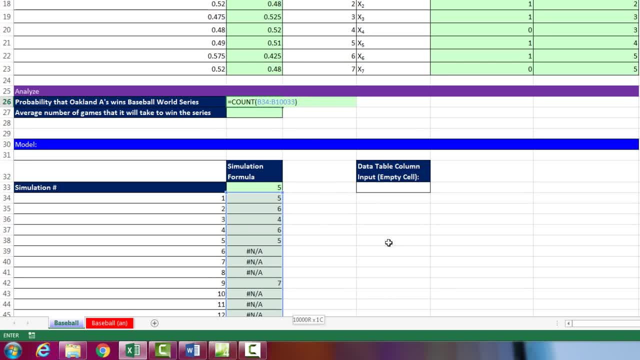 And I didn't count how many simulation values I have. so I'm going to divide by and I'm going to use ROW, because ROW tells me in a range how many rows there are. CTRL-SHIFT-DOWN-ARROW. 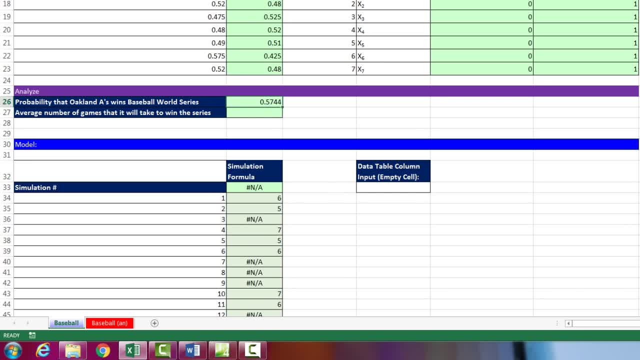 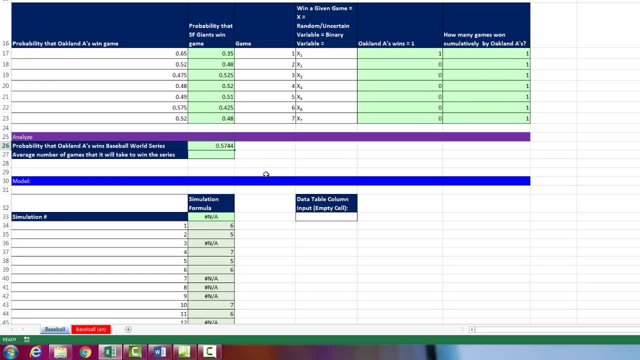 CTRL-BACKSPACE, close parentheses. And that formula will calculate the probability, based on this series of individual probabilities for winning games, that the Oakland A's will win the World Series. If I hit F9, you can see it's changing each time. 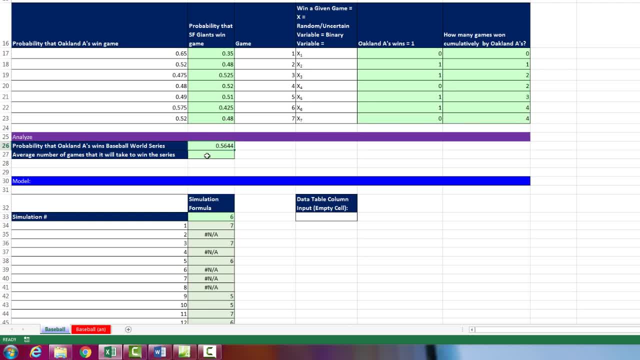 Now the next calculation is the average number of games it will take to win the World Series. Well, because we did our MATCH formula and now we can just take an average of all these. However, the errors will mess up a straight AVERAGE function. 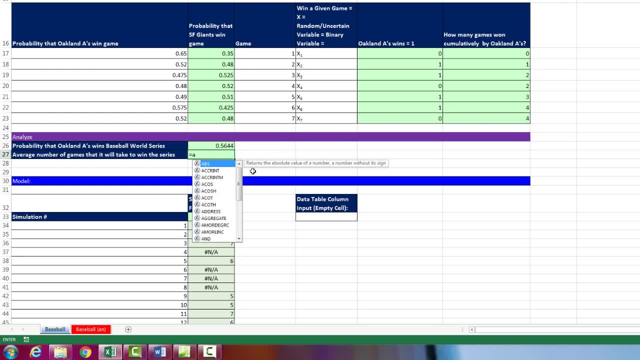 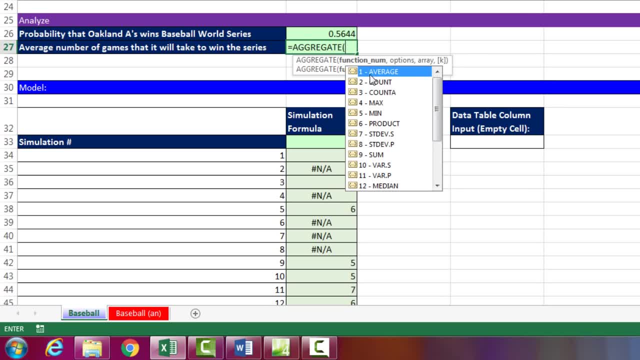 So, instead of using AVERAGE, like we've seen two times already in this chapter 11, we'll use the AGGREGATE function And we're going to use the first argument, number 1,, to tell it: please do the AVERAGE calculation. 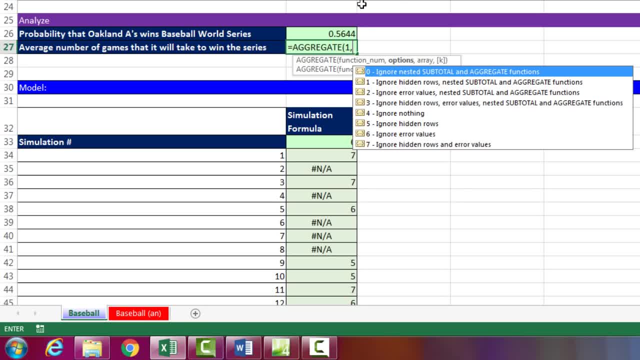 comma and unlike the other two times in this chapter, when we used AGGREGATE, it shows IGNORE NOTHING. but here we want to choose IGNORE ERROR VALUES. So this is a way of using AGGREGATE to calculate number 1 function, which is AVERAGE. 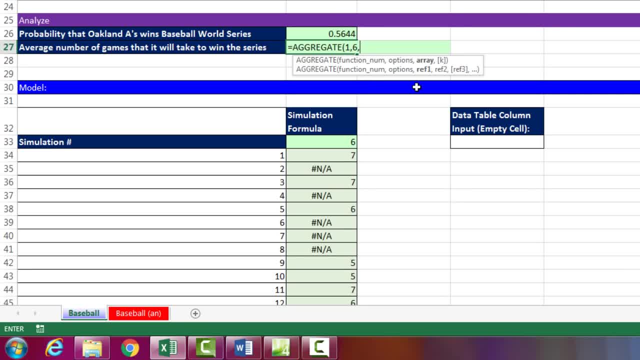 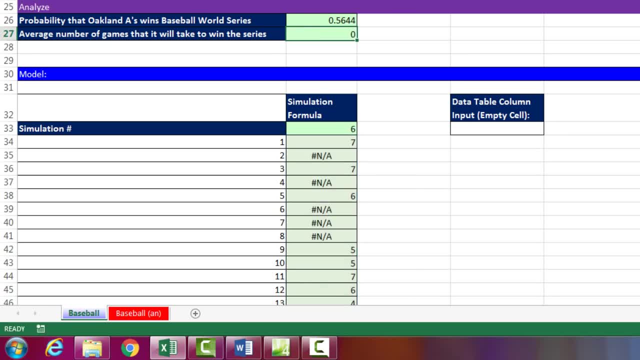 by IGNORING ERRORS. number 6 for options, comma and then the reference. click on the top cell, CTRL SHIFT, DOWN, ARROW, CTRL BACKSPACE, close parenthesis and ENTER. Now, if I hit F9,, F9,, F9,. 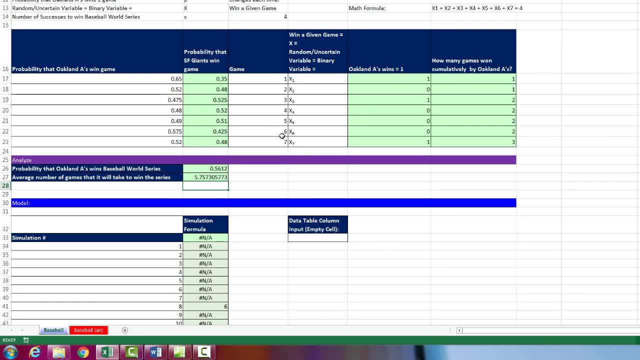 now we have our two calculations, based on individual probabilities that the Oakland A's will win a particular game against the Giants. We've calculated the probability that the Oakland A's will win and the average number of games. Wow, that was a lot for chapter 11,. 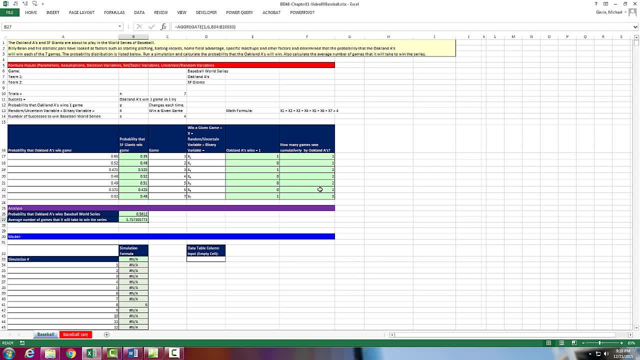 a lot of amazing tricks for simulation. We saw a bunch of different randomizing formulas for different variables that were based on particular probabilities distributions, and we saw that each time we used the data table feature and an empty cell to create our many simulated values. 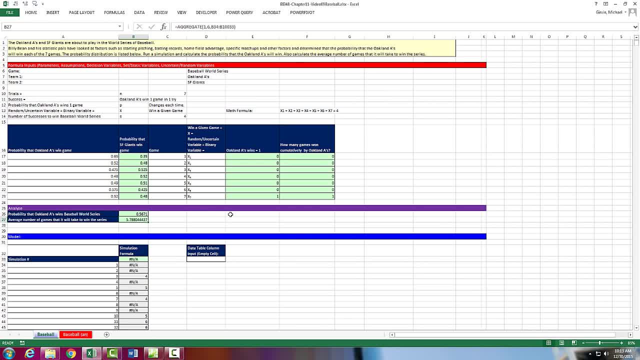 Alright, that's it for BI 348 class. We'll see you next. video series and video class. No matter what job you're in, and even if you're not working at all, there are some key analytical skills that everyone should know. These are skills that help you solve problems, create good solutions and take action. Become a better analytical thinker by the end of this video. Hi, I'm Jen. I'm here every. 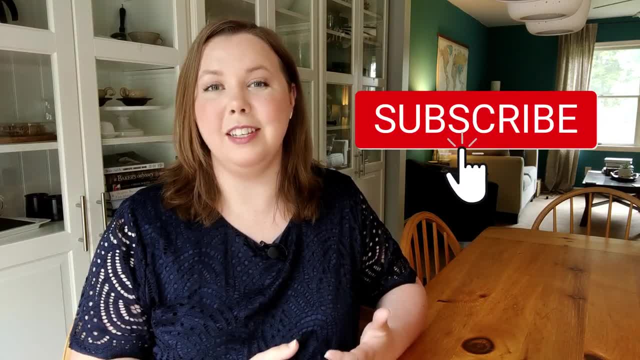 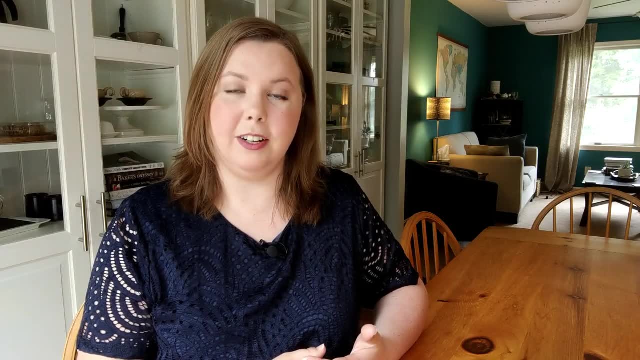 Thursday with videos related to analytics and the skills you need to be successful in the current workforce. In past analytical thinking videos, I've talked about the four steps of analytical thinking and I've also talked about how to further develop your skills in identifying problems and determining. 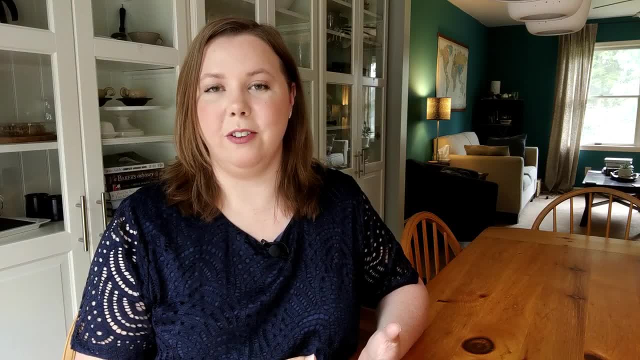 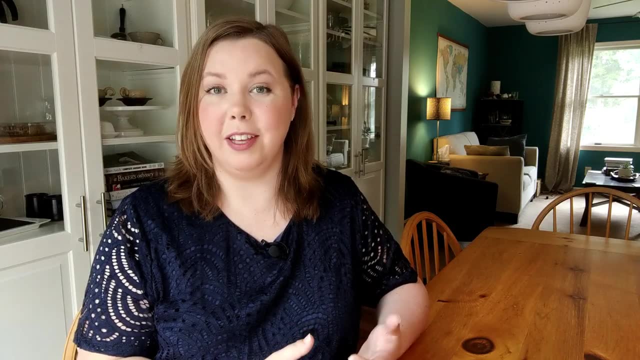 how you're going to solve them. Those are the first two steps of analytical thinking, and today we're going to focus a little bit more on the third and fourth steps of analyzing the problem and solving the problem. I'll link to the past two videos in case you haven't seen them. If you haven't watched them, I'd 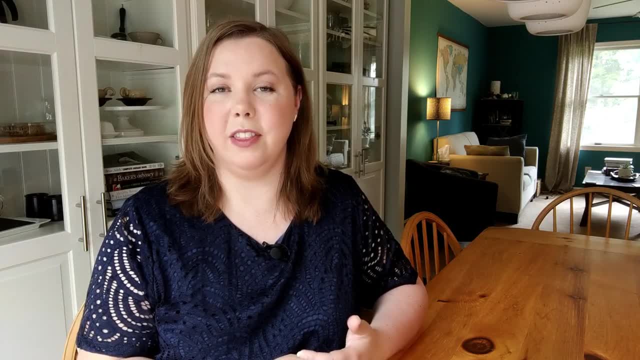 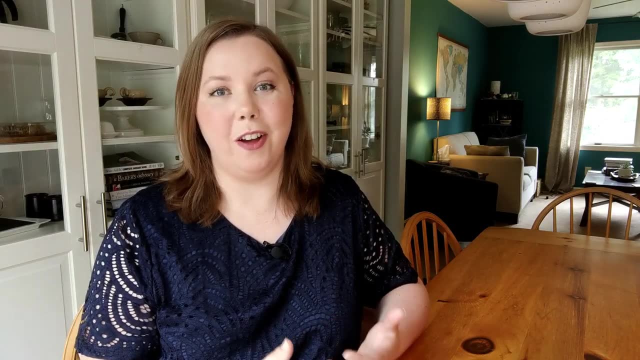 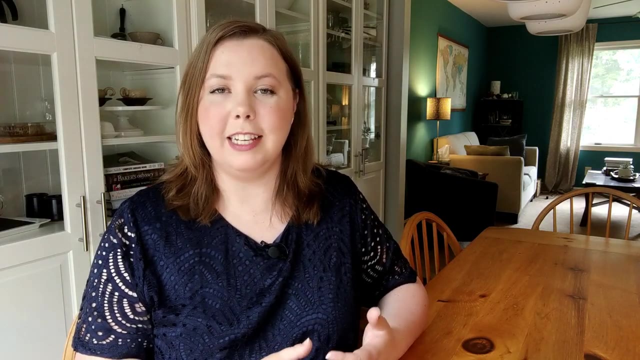 highly recommend at least starting with the four steps of analytical thinking so that you understand the problem a little bit better. Now let's look more at analyzing the problem and getting an answer or solving the problem. When it comes to analyzing the problem, one of the key challenges people face is that you will rarely have every piece of 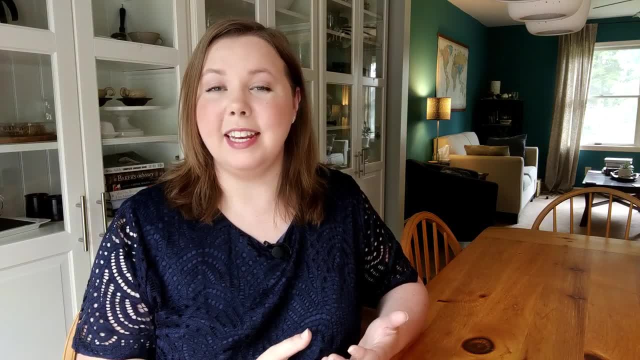 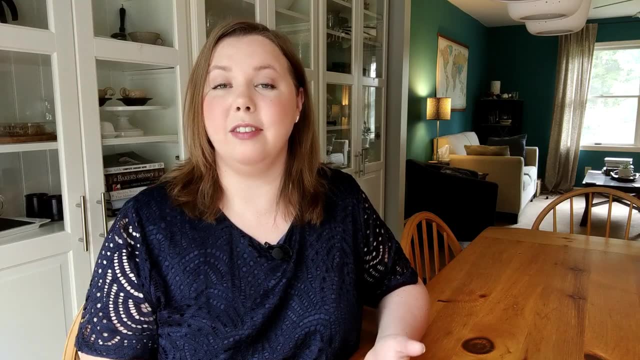 information that you need to be able to solve the problem, Whether the data doesn't exist or is just so difficult or time-consuming to get that it's not worth it. you're going to have to sometimes make assumptions. So what does analytical thinking say that we need to do to deal with this problem? Well, it's.